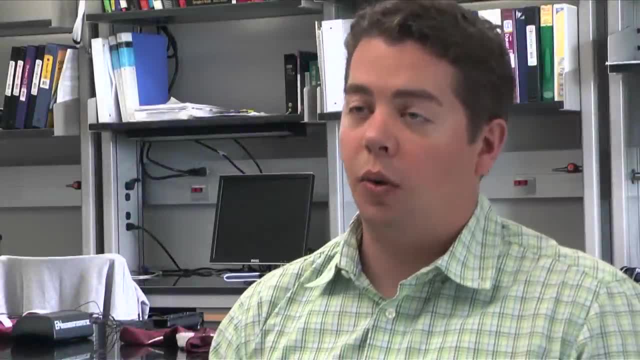 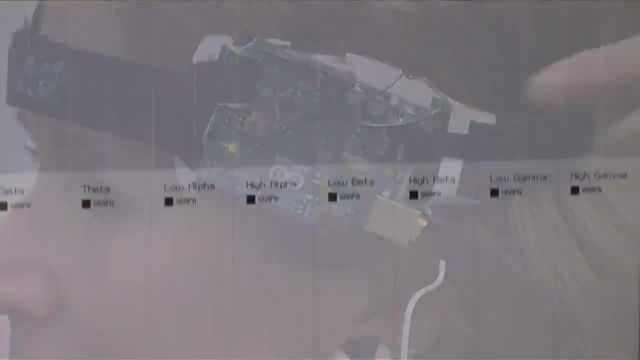 the cognitive efficiency study we're looking at ways to quantify how much information is communicated to a person and how reliably it is communicated, so that when they act on it, but also how much mental engagement it's requiring. So we're really interested in domains. where there's a very high level of communication between the two. So we're really interested in how much information is communicated to a person and how reliably it is communicated to a person. So we're really interested in domains where there's a very high demand for 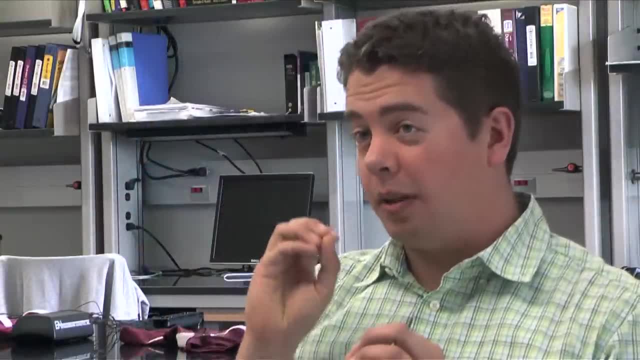 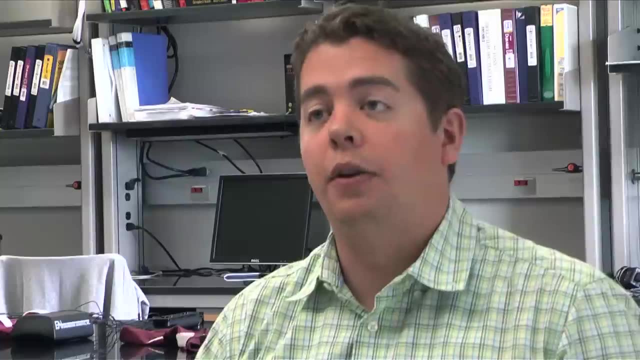 information processing resources. So it's very important that if we're going to communicate more information, that it's done in a minimally loading way. So we have a study that's looked at different ways to measure both the informativeness of a message as well as that cognitive engagement. 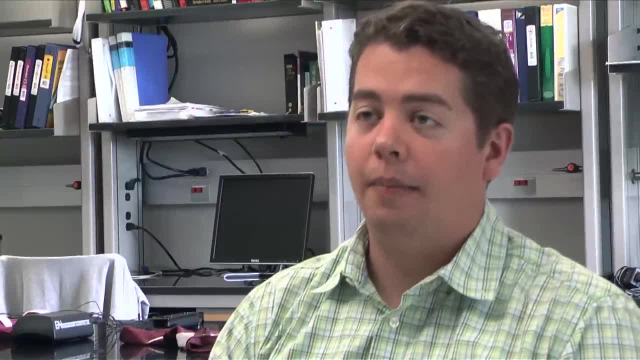 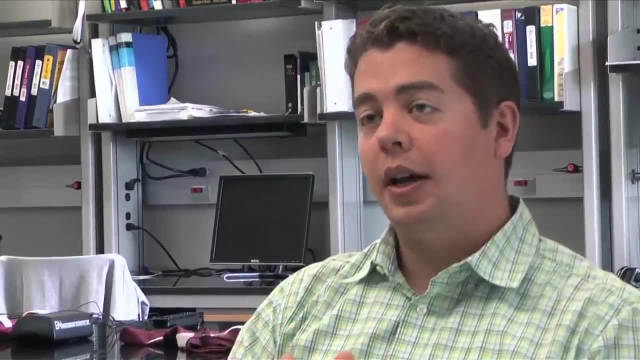 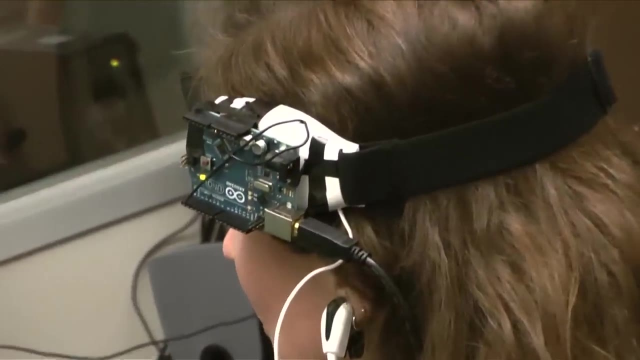 And some of the ways we've looked at cognitive engagement include subjective measures, some standardized scaling, but maybe some more interesting ones. We use performance measures and we look at physiological measures. So we're looking at electrical brain activity, the electroencephalography, skin conductance and a number of other measures that we're 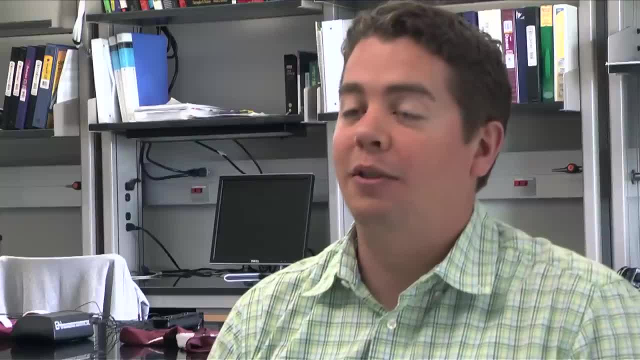 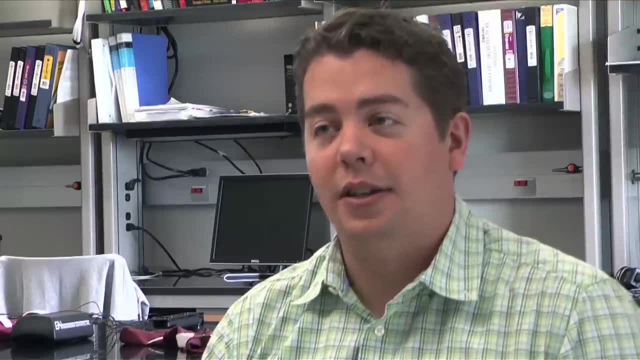 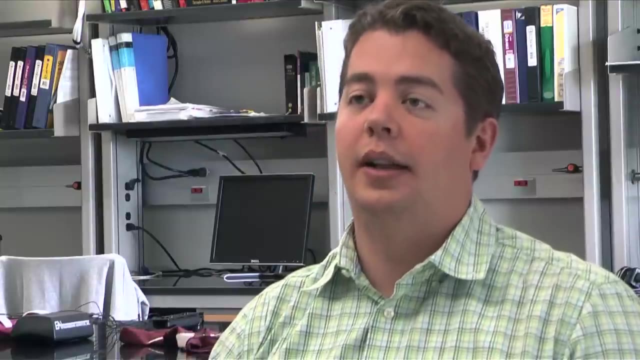 considering. So we have equipment to be able to measure those things and we've been looking at some very simple displays that just use very fundamental display dimensions and looking at how this affects the informativeness- people being able to receive the information from the message- as well as how engaging it is for their cognitive resources. 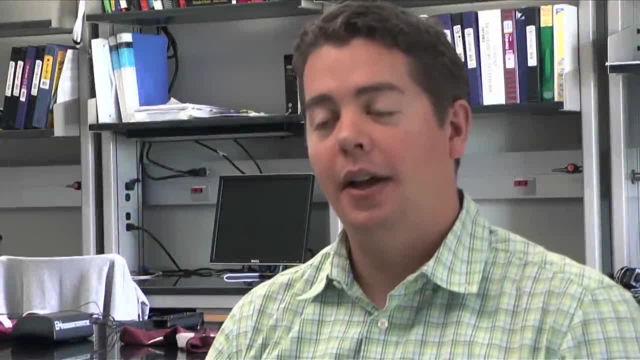 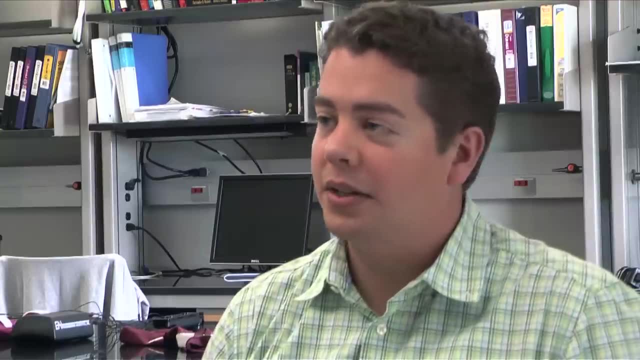 We're particularly interested in the sense of touch as a channel other than vision and audition. that really has a lot of potential but hasn't been explored very fully in a lot of domains. Now, the sense of touch has some unique properties. It tends to be one that 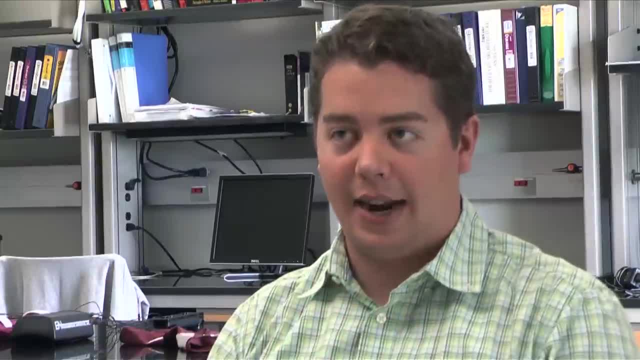 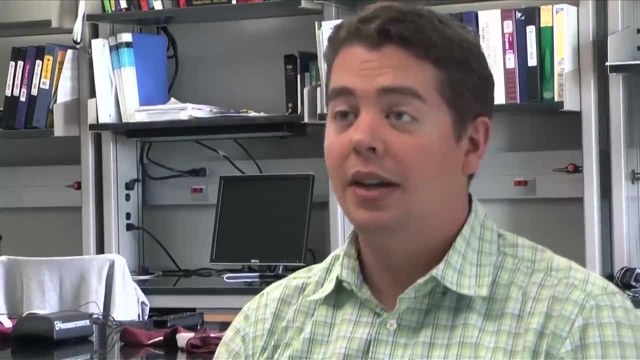 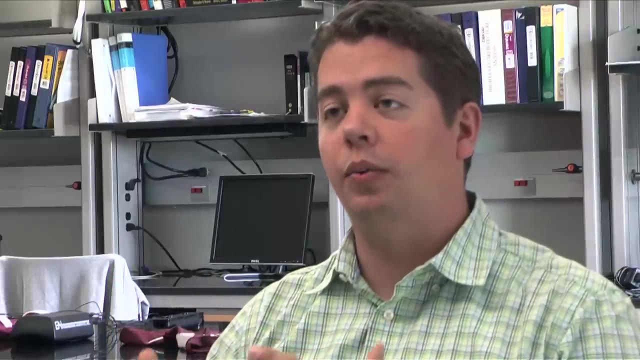 we can sense a tactile signal from any direction, regardless of where our attention is oriented. We call it an omni-directional sense, just like audition. But unlike audition it tends to be very well coordinated with our motor system. So if you need somebody to do a movement, 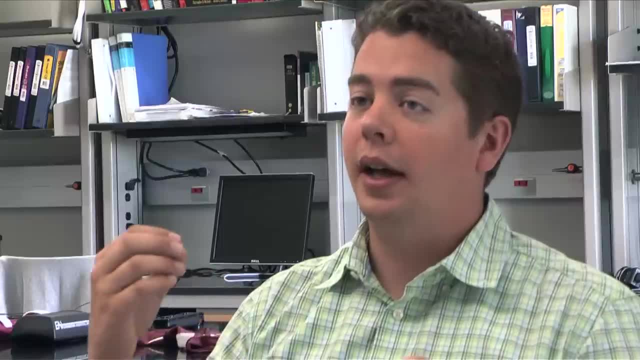 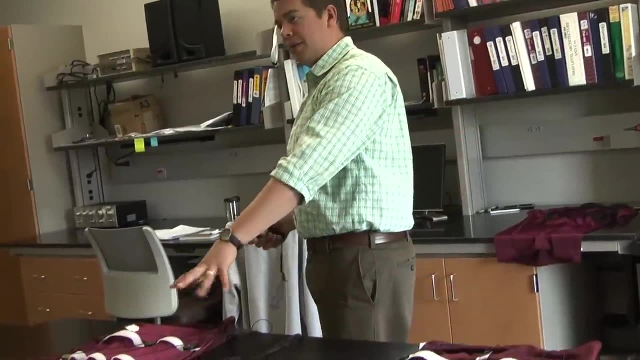 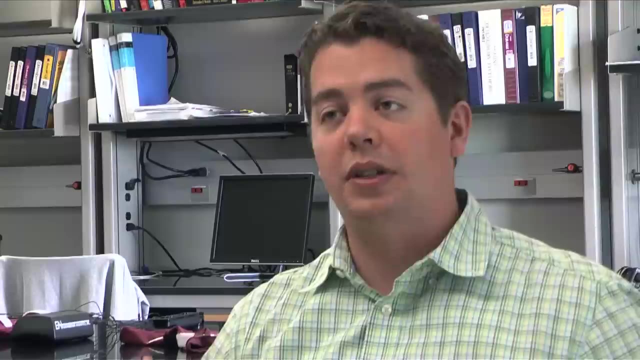 one of the best ways to do that is to relay the information via a particular location being vibrated on that person's body. So we've developed a system to help us do this in a very we call it closing the loop from somebody sending a message to a person receiving it, if the message is some sort of 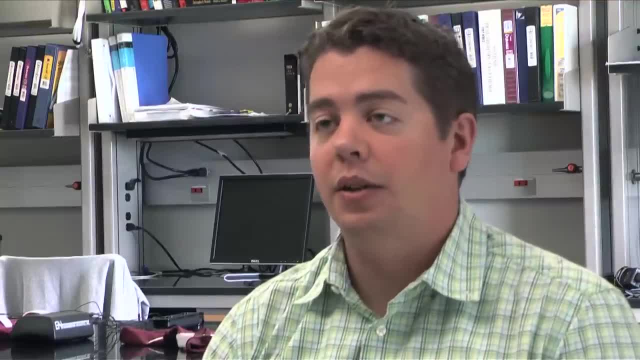 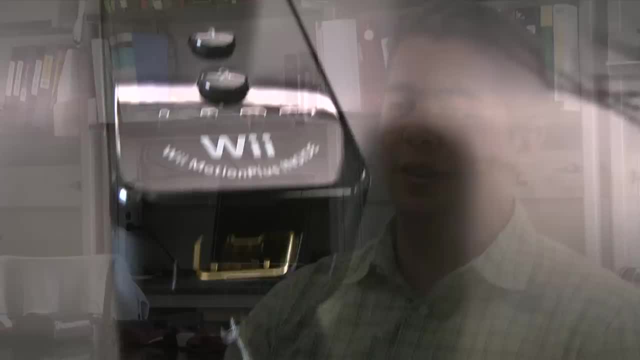 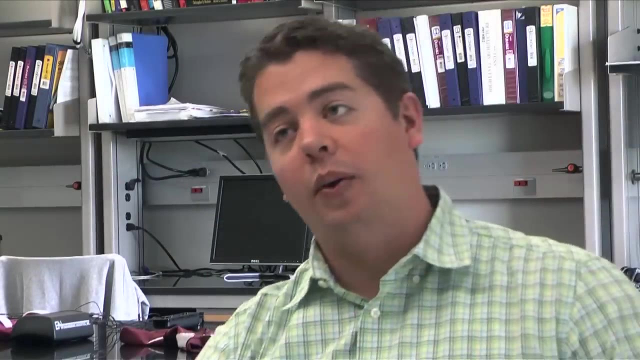 motor direction. So we have a display that uses a gestural-based input. So we use a gyroscopic controller, a Nintendo Wiimote that we've repurposed as a gesture controller, And we have a commander who can send messages by waving this controller. so it's a very 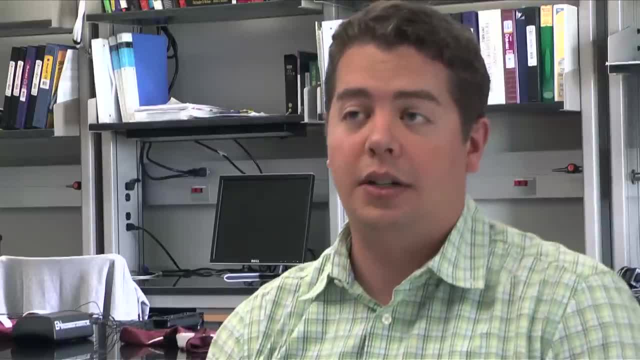 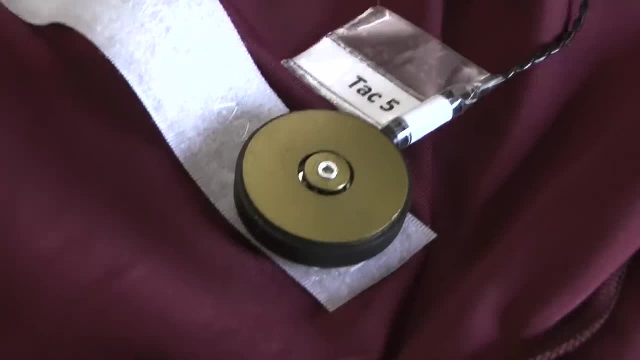 intuitive way to direct somebody, give somebody directional instructions, And then we've mapped that to patterns of vibrations that would be presented on a receiver's almost like a shirt display. So we have these vibrators embedded in the shirt and they can receive this pattern of. 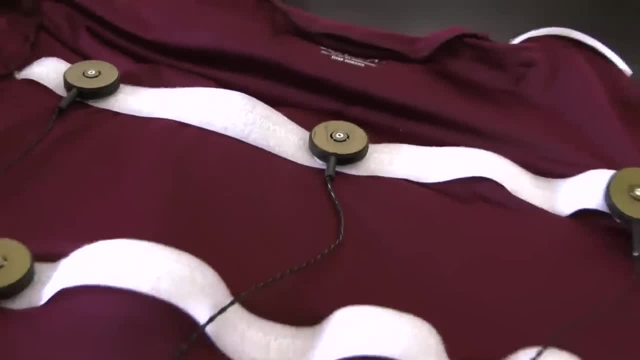 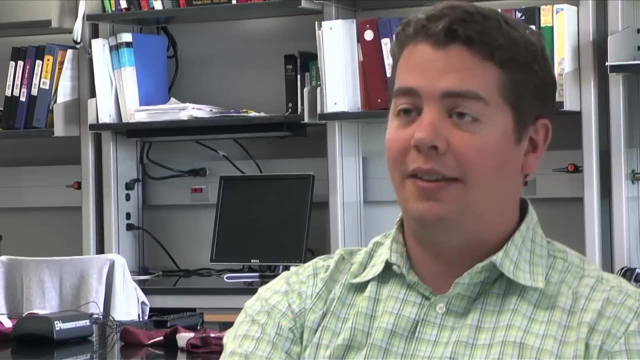 vibrations, And the idea is that we can direct someone in a very efficient way, because we're shortening the amount of time it takes the sender to send a direction, because they can just gesture. They don't have to think about how to say it or how to visually orient somebody. 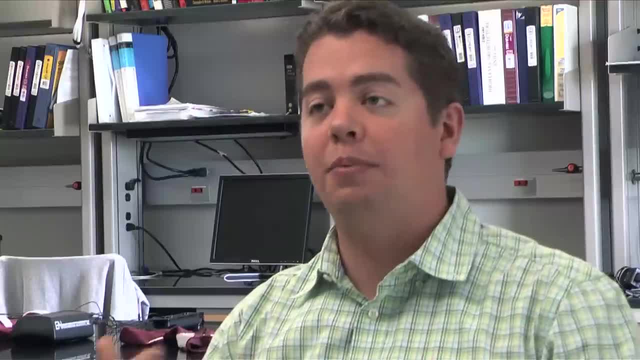 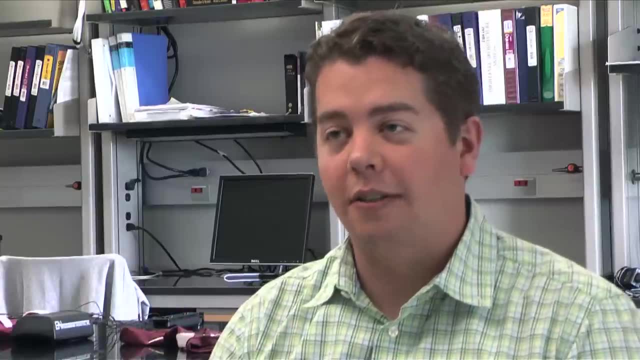 And then the receiver. The receiver acts very intuitively that they can almost perceptually respond to the vibration displays if it's directing them. And we're also looking at some other additional questions. How far can we push this display? So how much information can we reliably relate with the sense of touch? 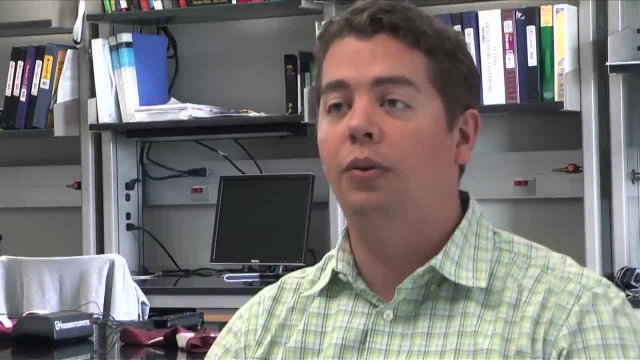 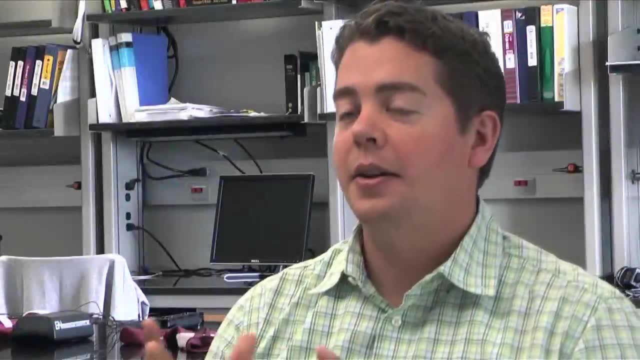 And can we find a way to have two communicators develop their own intuitive way to use the system? So there are a number of applications we can look at there, If you can think of any domain where you might have to send a message to somebody. 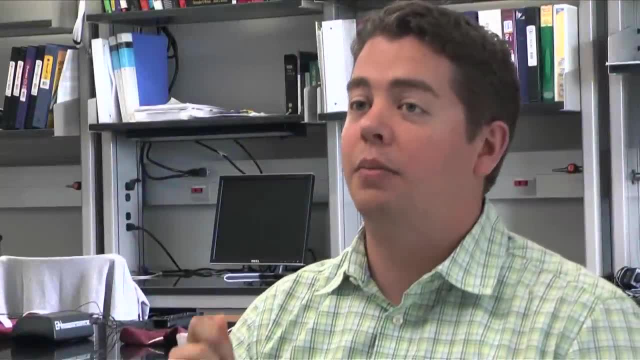 I'm going to go ahead and do that. I'm going to go ahead and do that If you can think of any domain where you might have to send a message to somebody very quickly and have them respond by physically moving as quickly as possible. 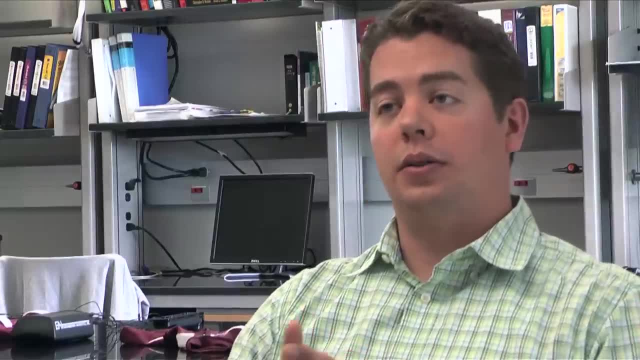 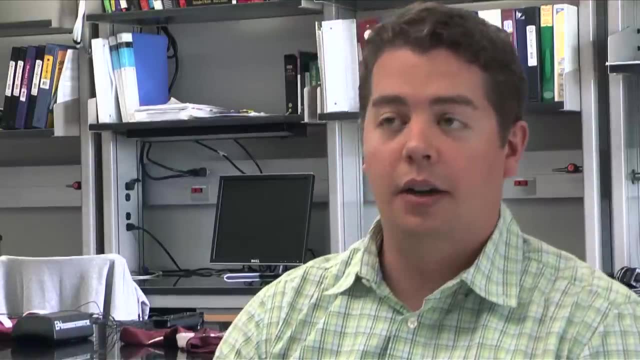 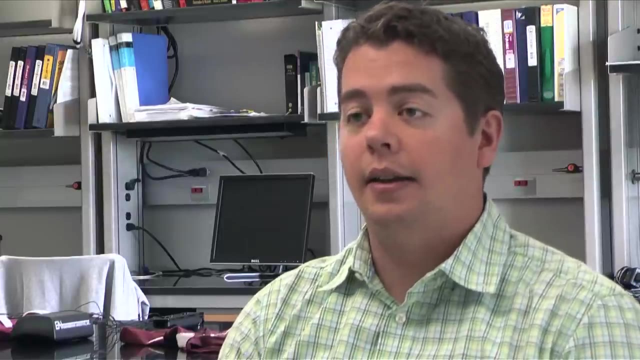 So a great example would be firefighting. You have somebody who is moving throughout a dynamically changing environment, dynamically changing threat levels in different locations. Another great example are military applications- dismounted soldiers, maybe in a battlefield scenario. And another example we like to talk about are leisure sports.